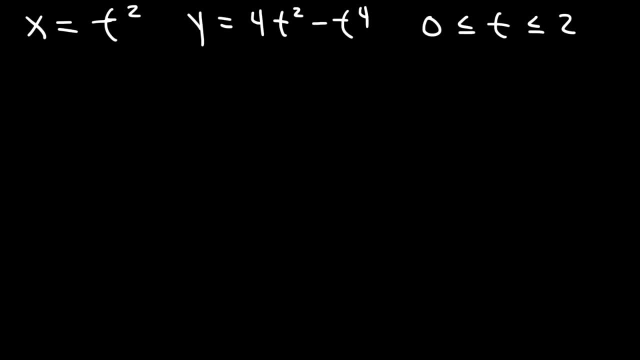 And we want to find the area under the curve where t is bounded between 0 and 2, and it's going to be between the curve and the x-axis. So what formula should we use? Now, let's say, if we have some function where y is equal to f of x and we wish to find the area under the curve from a to b? 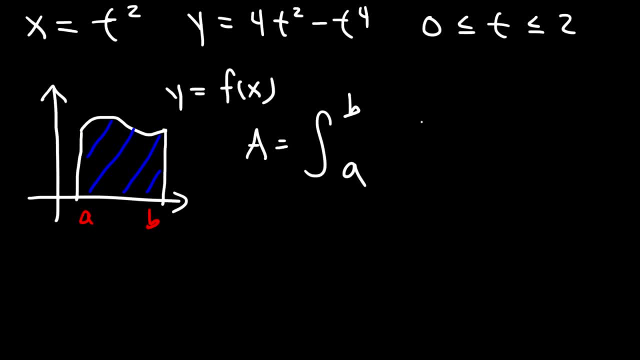 The area under this curve will be the integral from a to b of f of x, dx. So in this case we can see that y is f of x. so we can say that the definite integral from a to b, y, dx will give us the same area. 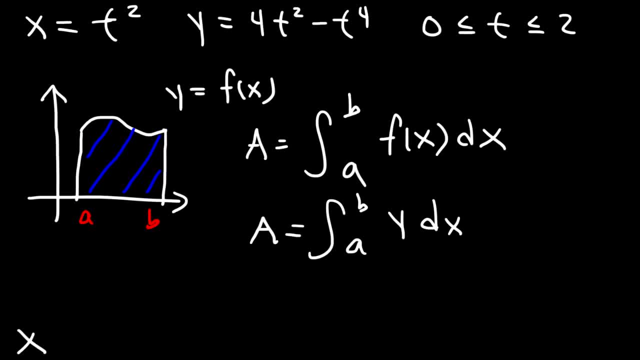 Now let's say that x- let me write it down here- is equal to f of t, and let's say that y is g of t. In that case we can replace y with g of t. Now if we have some function where y is equal to f of x and we wish to find the area under the curve between 0 and 2, and it's going to be between the curve and the x-axis- 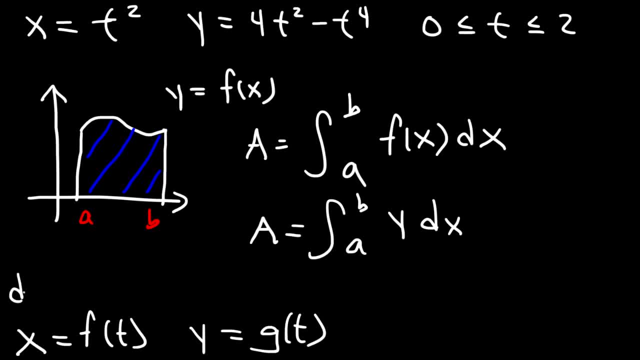 So in this case we can see that y is f of x. so we can say that the definite integral from a to b, y, dx will give us the same area. Now if we differentiate both sides, we can get the differential. dx is equal to f prime of t times dt. 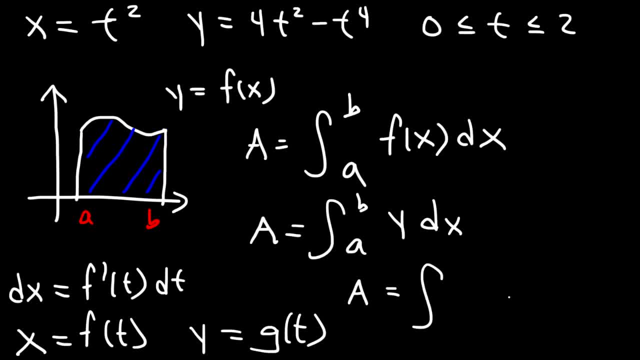 So therefore we can say that the area is going to be the integral of g of t. so we replace the y with g of t and then, replacing dx with f, prime of t, dt, we get this expression And the limits of integration will change from a and b to alpha and beta, where alpha and beta represent t values. 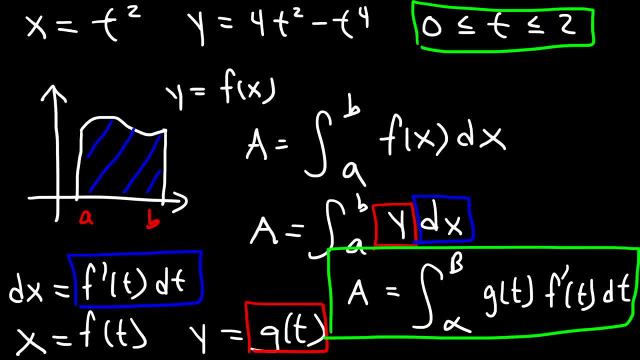 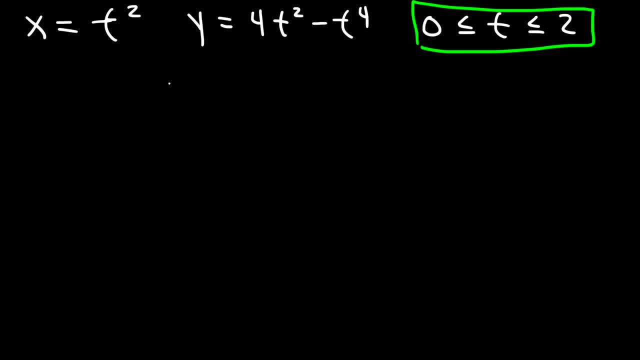 And so this is the formula that we want to use when finding the area under a curve of a parametric function. So let's begin by graphing this parametric function. Let's make a table. So we're going to have t, x and y. 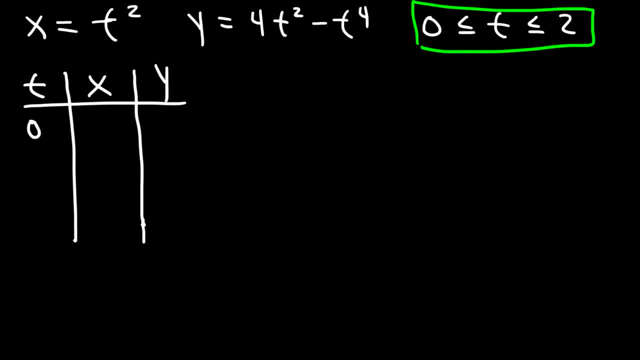 So let's start with: t equals 0.. When t is 0,, we can see that x is going to be 0, and y is going to be 0 as well. Now, what about when t is 1, and when t is 2?? 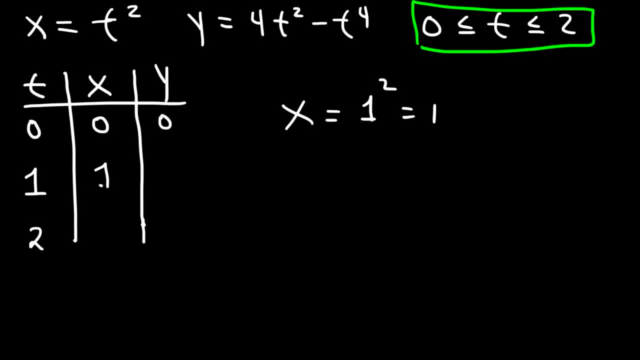 So x will be 1 squared, which is 1.. And when t is 2,, x is going to be 2 squared, Which is 4.. Now let's find the y values. So when t is 1,, this is going to be 4 minus 1, which is 3.. 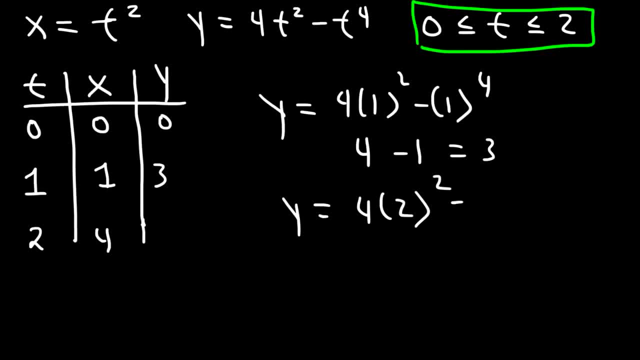 And when t is 2,, 2 squared is 4,, 2 to the 4th, power is 16,. 16 minus 16 is 0.. So we're going to have: t is 0.. So y is 0.. 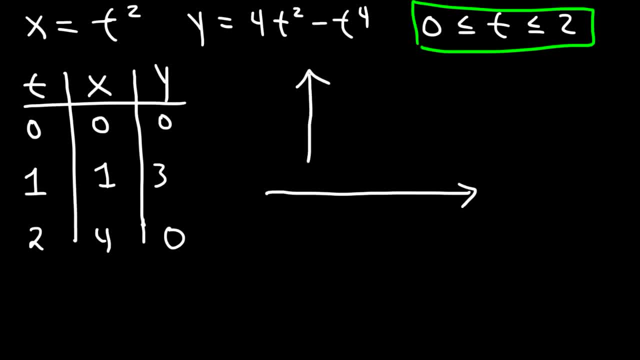 Now let's go ahead and plot the points. So, when x is 0, y is 0. And when x is 1, y is 3. And when x is 4, y is 0. Now it looks like we need a few more points. 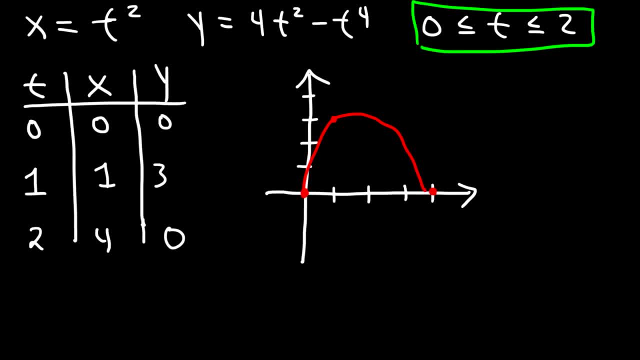 Because if we graph it, it's going to look something like this: But let's just see what's happening in the middle. So, when x is 2, what is y? Using this equation, when x is 2,, 2 is equal to t squared. 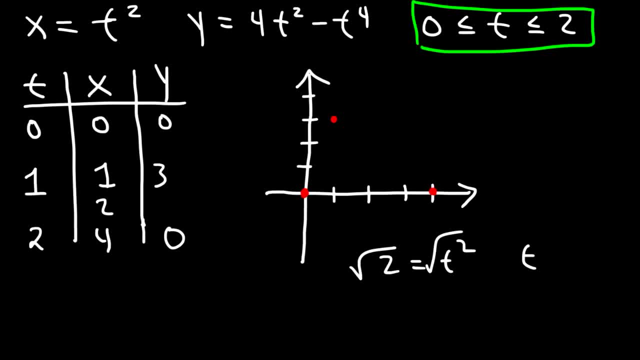 And t is going to be the square root of 2.. Now let's go ahead and plug that value into this equation. So y is equal to 4t squared. t squared is 2 minus t to the 4th power. So that's the square root of 2 raised to the 4th power. 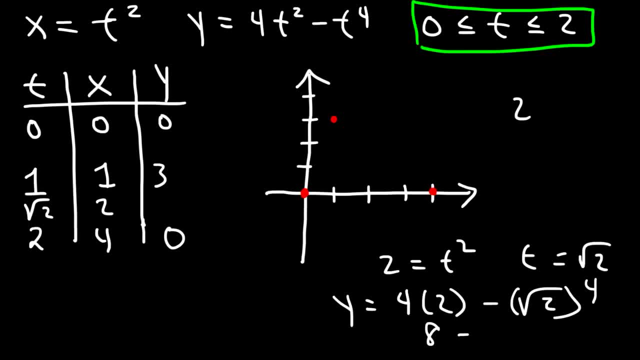 So this is 8.. And the square root of 2 is basically 2 to the 1 half Raised to the 4th power, 1 half times 4 is 2, so that becomes 2 squared, which is 4.. 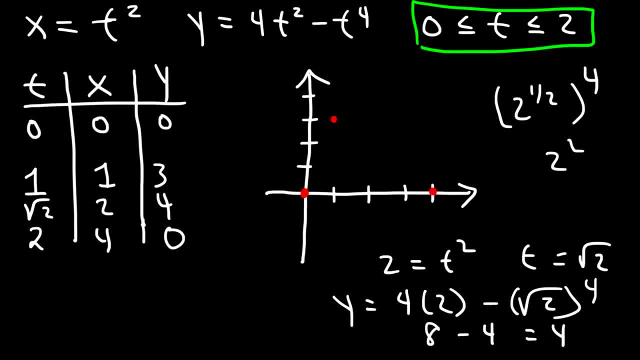 So y is 4.. So when x is 2, y has a value of 4.. Now what about when x is 3?? When x is 3, t is going to be the square root of 3.. So now we need to calculate y. 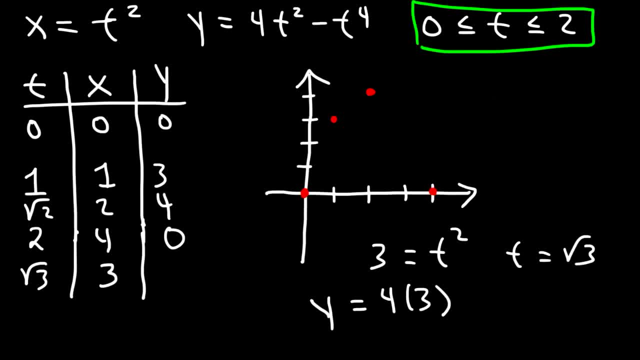 So it's going to be 4t squared and t squared is 3, minus t to the 4th, Or the square root of 3 raised to the 4th power. So 4 times 3 is 12.. 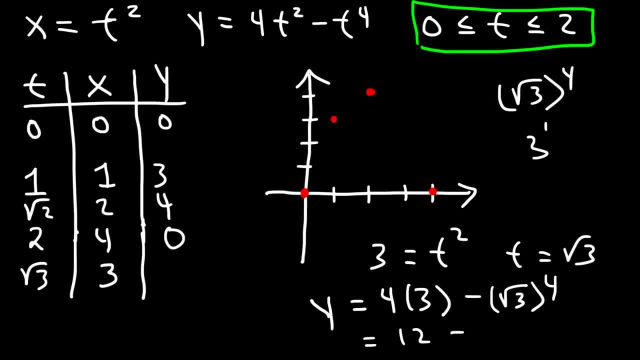 And the square root of 3 to the 4th power, That's 3 to the 1 half Raised to the 4th power, Which is really 3 squared, And 3 squared is 9.. 12 minus 9 is 3.. 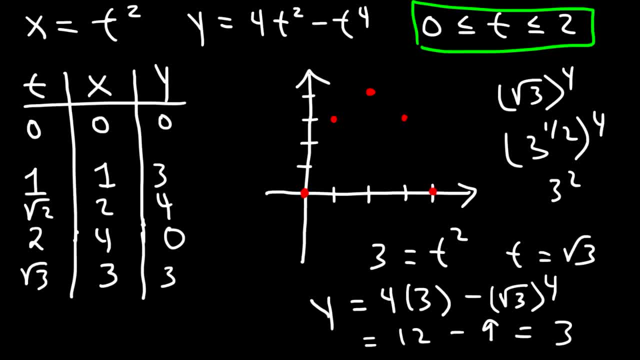 So when x is 3, y is 3.. And so the parametric function looks like this. Now let's calculate the area under the shaded region between these two t values, From 0 to 2.. Or when x goes from 0 to 4.. 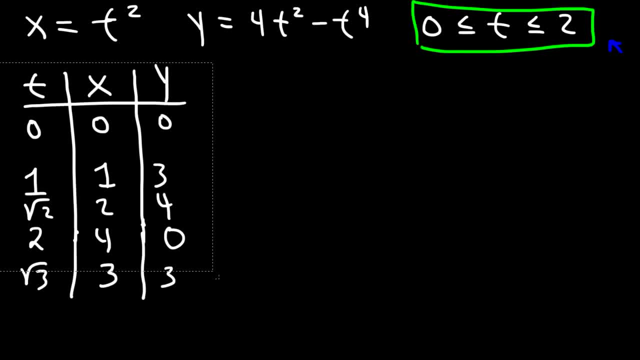 So let's begin with this formula. The area is going to be the integral from alpha to beta. g of t times f, prime of t, dt. So we defined x to be f of t. So therefore, f of t is t squared And g of t, we define that to be y. 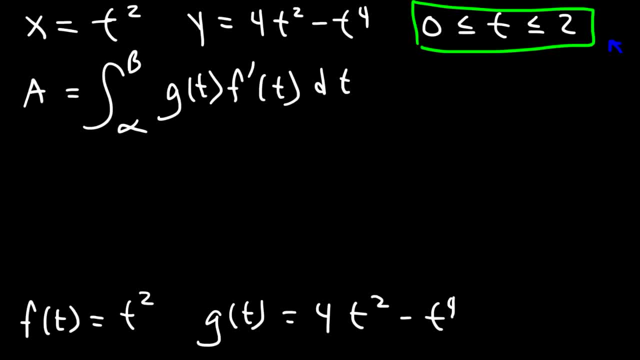 So that's going to be 4t squared Minus t to the 4th power. Alpha is 0.. Beta is 2. Based on the values that we see here. So let's replace g of t With 4t squared. 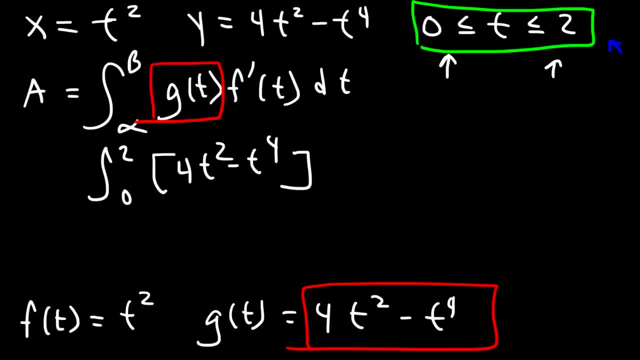 Minus t to the 4th power And then f prime of t. If f of t is t squared, f prime of t is 2t, And then we have dt. So let's distribute 2t to what we see here. 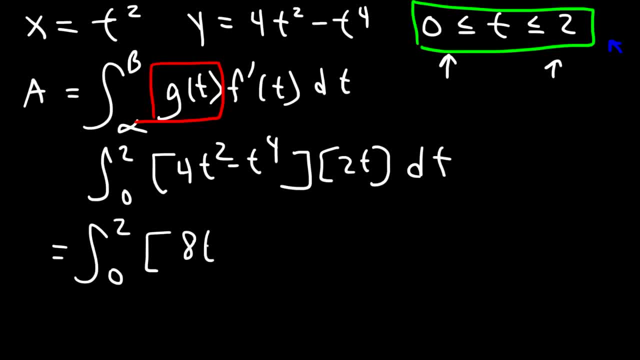 4t squared times 2t, That's going to be 8t to the 3rd power And t to the 4th times 2t, That's going to be 2t to the 5th power. 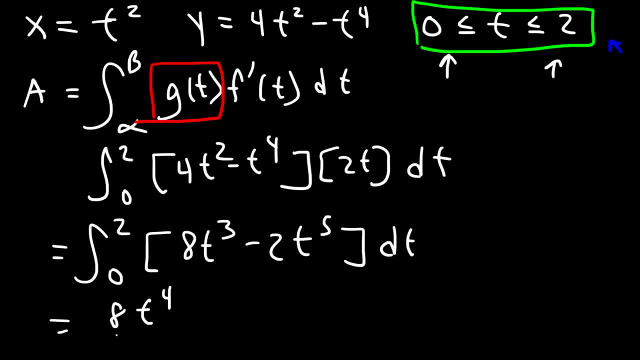 The antiderivative of t cubed is going to be t to the 4th power over 4.. And the antiderivative of t to the 5th Is t to the 4th power And t to the 6th over 6.. 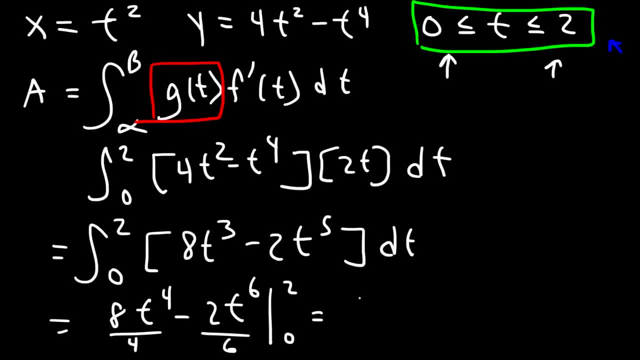 And let's evaluate it from 0 to 2.. So if we plug in 2.. 8 over 4 is 2.. So that's going to be 2 times 2 to the 4th power, And then 2 over 6. we can reduce that to 1- 3rd. 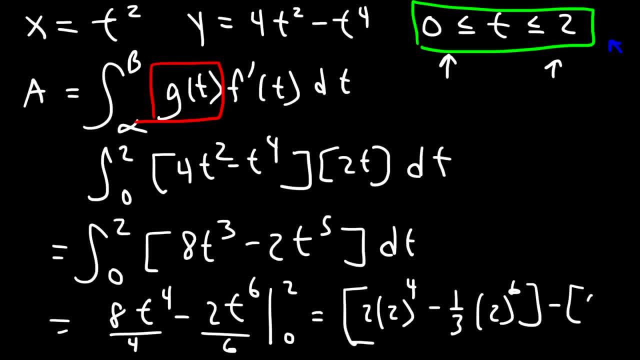 And then times 2 to the 6th power And if we plug in 0, the whole thing is 0. So let's make some space, Let's make some space. So the area is going to be 2 to the 4th power. 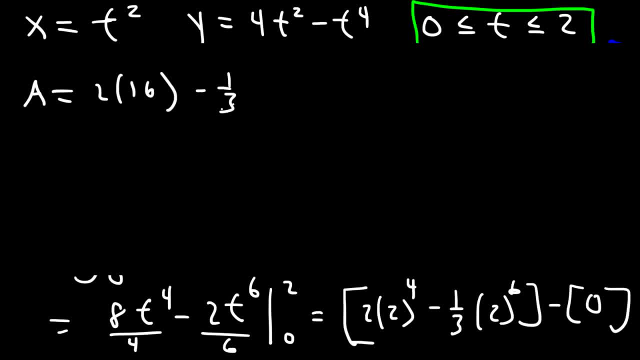 Which is 16. And 2 to the 6th power, That's going to be 64. So we have 32 minus 64 over 3.. Now we need to get common denominators. So let's multiply 32 by 3 over 3.. 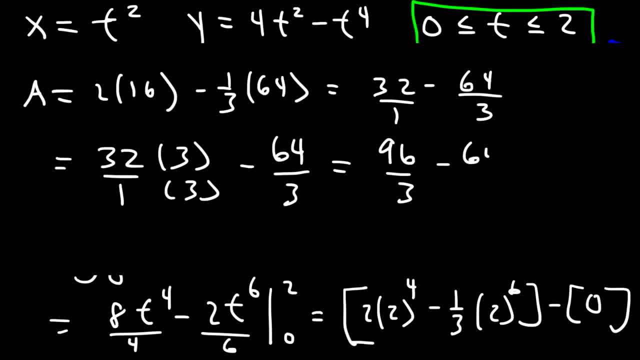 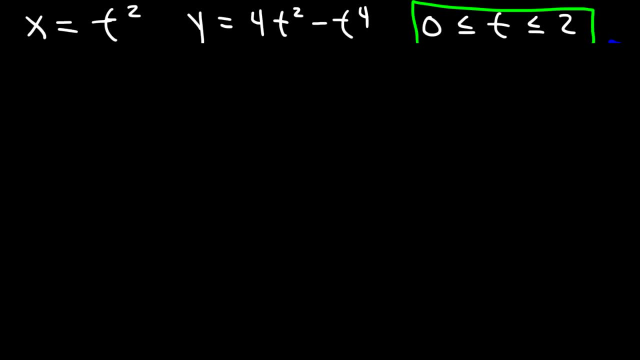 And that's going to be 96 over 3.. Minus 64 over 3.. 96 minus 64 is 32.. So the area is 32 over 3.. Now let's see if we can confirm that answer So using these two parametric equations. 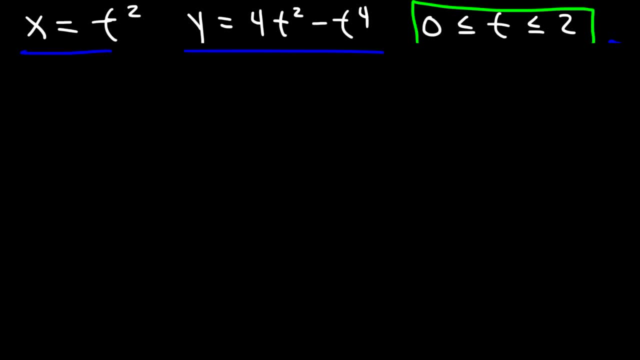 Let's write a function 4y of x, So x is equal to t squared. If we square both sides, that means that x squared is equal to t to the 4th. So we can replace t squared with x And we can replace t to the 4th with x squared. 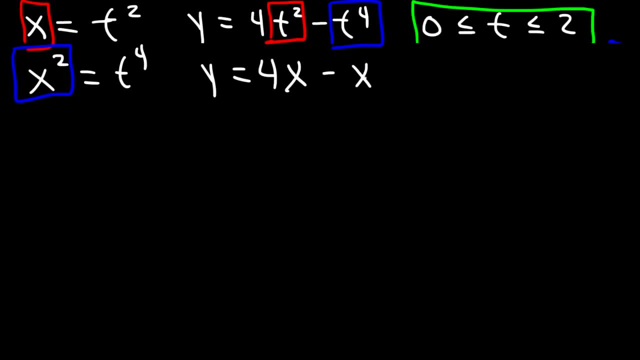 So we have: y is equal to 4x minus x squared. So now we have y as a function of x. So we can say that f of x, which is y, That's 4x minus x squared. Now let's convert the t values to x values. 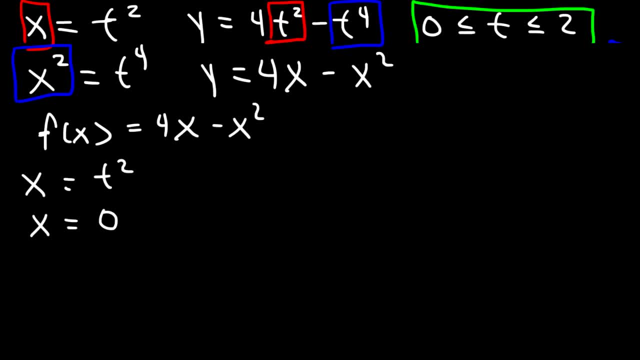 So x is equal to t squared, And when t is 0,, x is 0.. And when t is 2,, x is 4.. So let's calculate the area from 0 to 4.. f of x, dx, The antiderivative of. 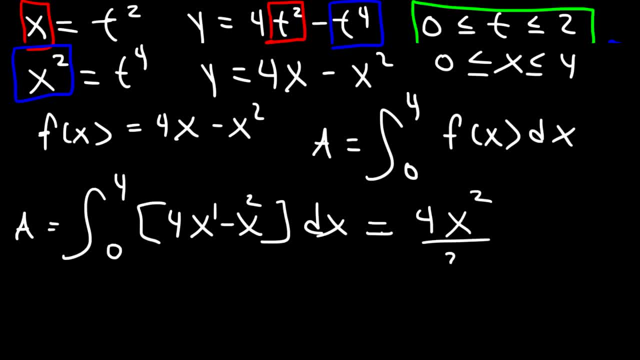 x to the first power is x to the second, power over 2.. And the antiderivative of x squared is x cubed over 3.. Let's evaluate it from 0 to 4.. So let's plug in 4.. 4 divided by 2 is 2..